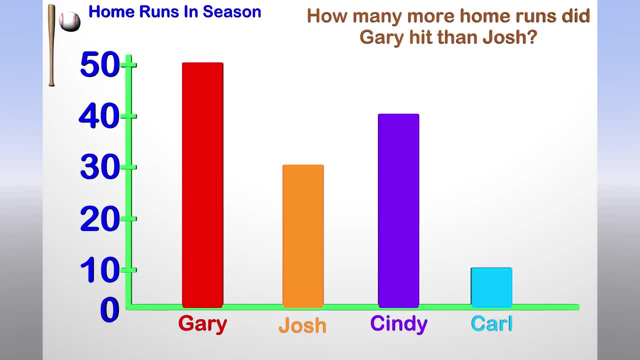 The first question we have is: how many more home runs did Gary hit than Josh? We know Gary had 50 and Josh had 30. We need to know how many more home runs Gary had than Josh. How do you think we can solve this problem? We can solve this question by using subtraction: Gary had 50 and. 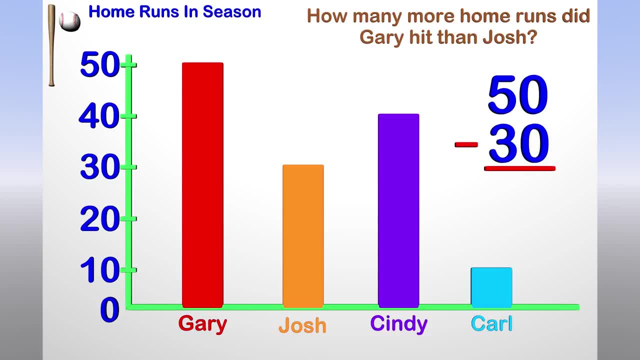 we subtract the amount Josh had, which is 30.. What is 50 subtract 30?? The answer is 20.. Gary had 20 more home runs than Josh. Great job, Using the bar graph, we solved the problem. Here is another problem that we need to solve: The. 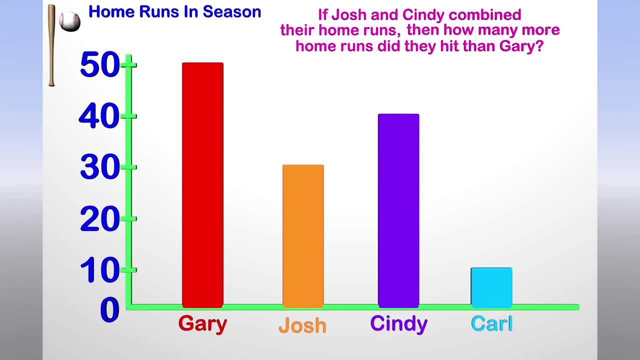 problem says: if Josh and Cindy combined their home runs, then how many more home runs did they hit than Gary? This question is a little bit harder because there are two parts to solve. How would you solve this problem? To solve this problem, the first step is to 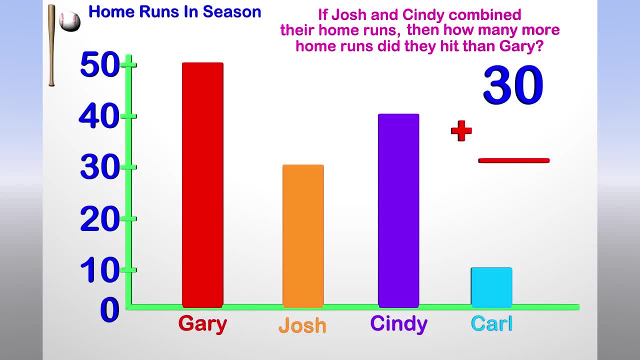 Josh and Cindy's home runs. Josh had 30 home runs and Cindy had 40. What is 30 plus 40? 70 home runs combined. Great job, That was the first part of the question. Now we need to know how many more home runs they hit than Gary. We know that combined. 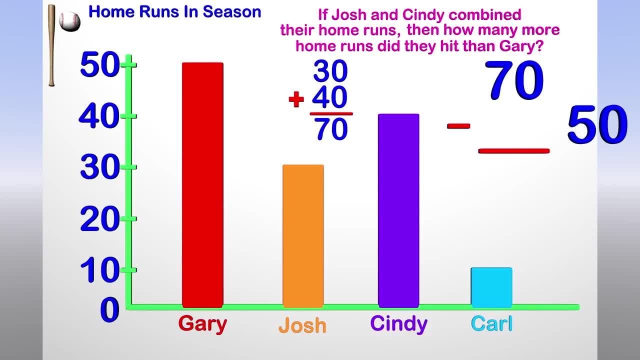 they hit 70, so we need to subtract the home runs Gary hit, which is 50.. What is 70 subtract 50?? The answer is 20.. With their home runs combined, Josh and Cindy had 20 more than Gary. Great job, guys. You did amazing and you sure know how to use a bar graph Now. 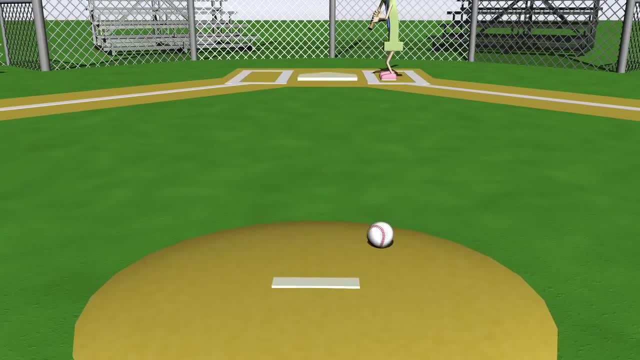 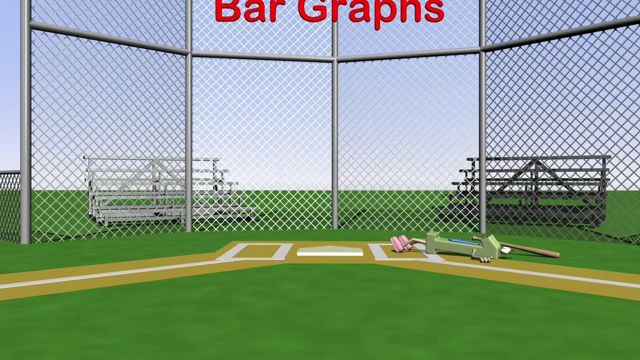 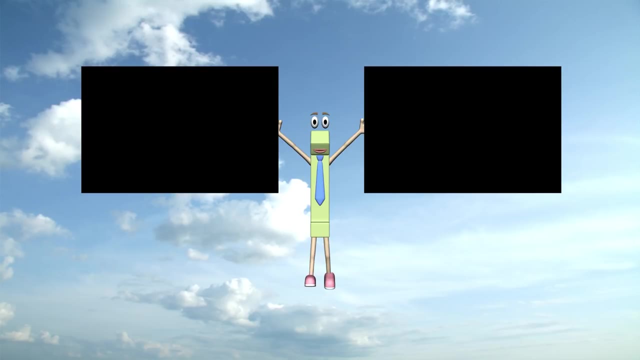 let's see how you do with pitching the ball to me. All right, give me your best throw. Whoa, that was a really good throw, Ouch. Hey guys, you have a few options here. If you want to subscribe, click the red button below. If you want to watch more awesome stuff, you can click the video on.